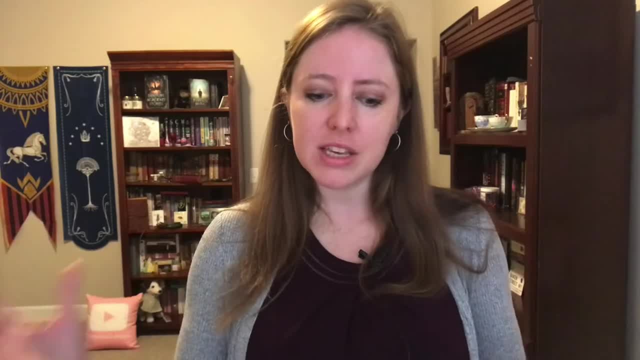 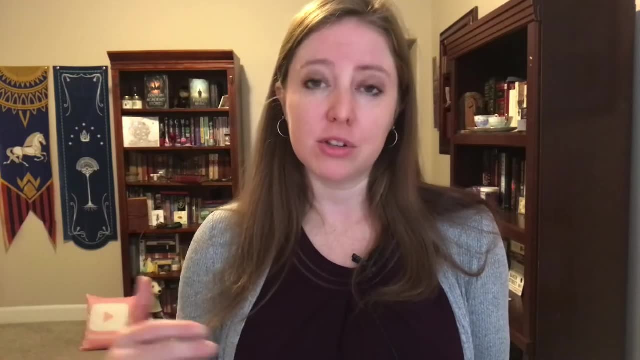 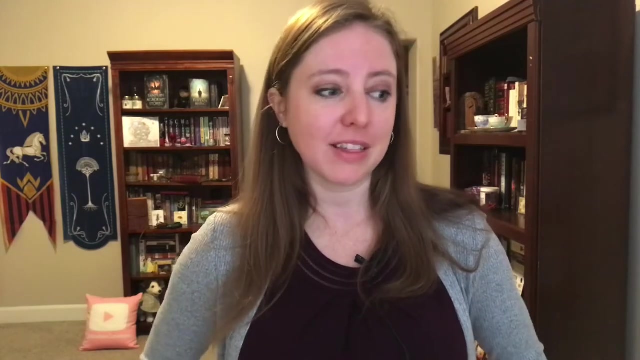 the Irish at the time, And so he satirically suggests that, in order to make money, the poor Irish could sell their one-year-old babies to be eaten and used for various like lampshades and things like that. It's really grotesque, but that is how a lot of satire tends to go. So how can you? 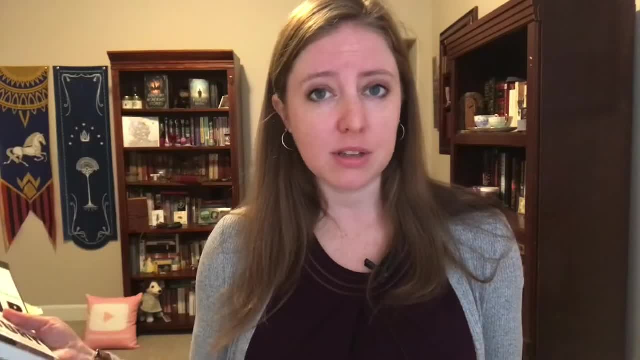 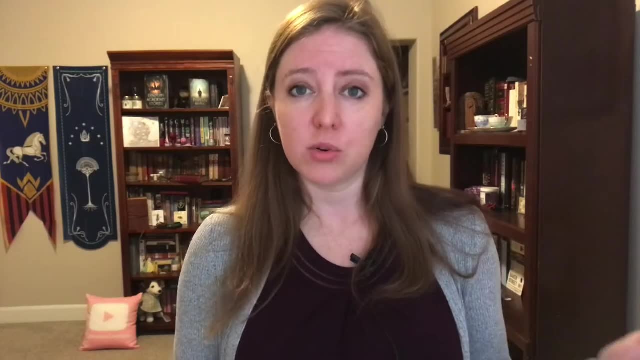 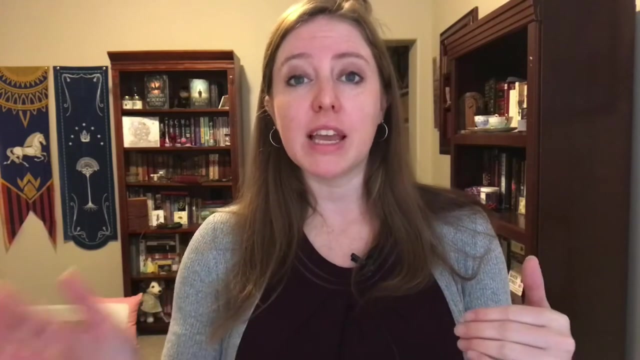 distinguish satire from other types of writing. I found that it's not always the easiest to pinpoint if something is serious or satire. One of the ways that you can tell is hyperbole. Satire almost always has this inflated lampshade. It's either loaded language which is emotionally charged, kind of words that 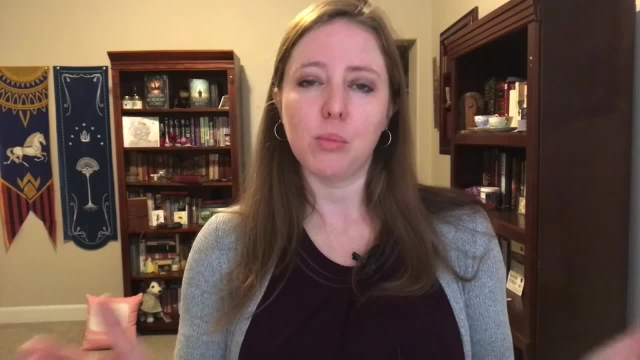 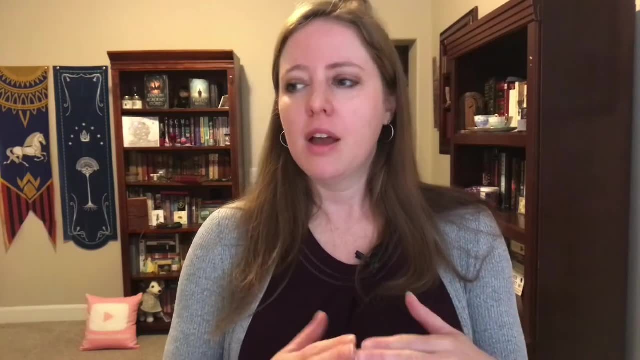 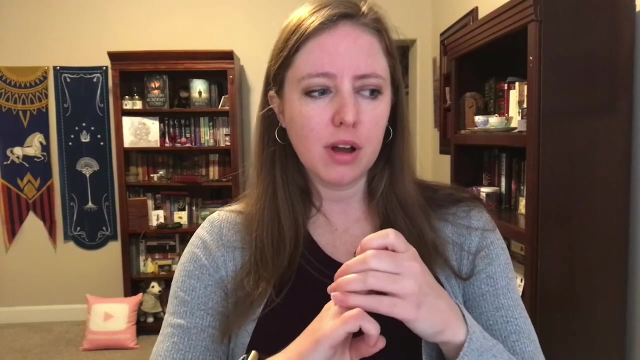 make you stop and go that's not quite matching up with what you're talking about, or just straight-up hyperbole, which is extreme exaggeration. So if you spot one of those things, then it is very possible that you're looking at satire If you come away with the impression that something really ought to be. 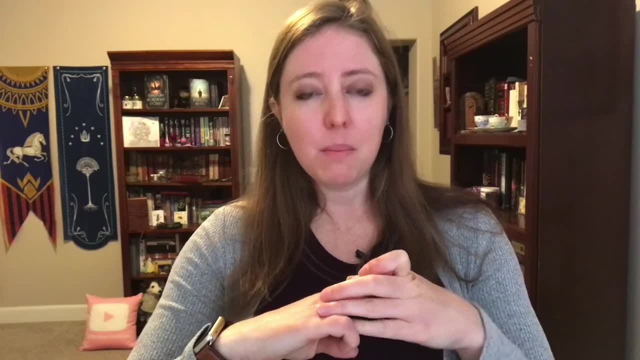 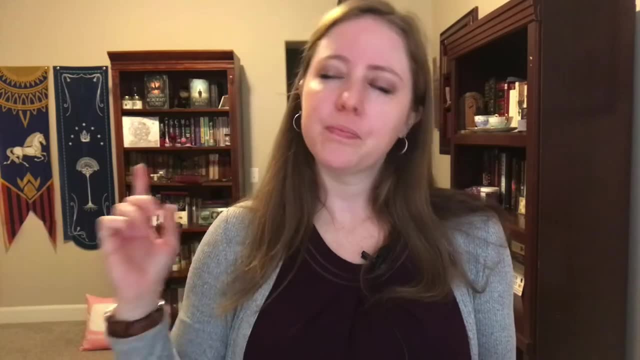 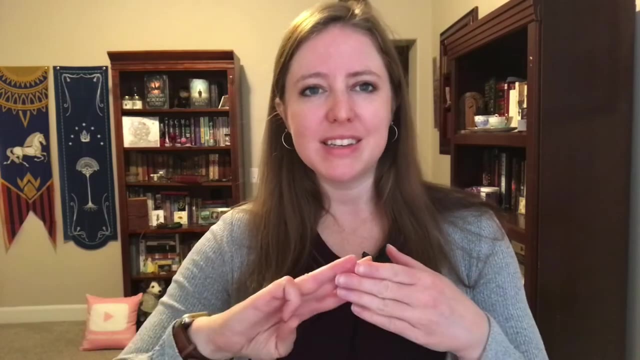 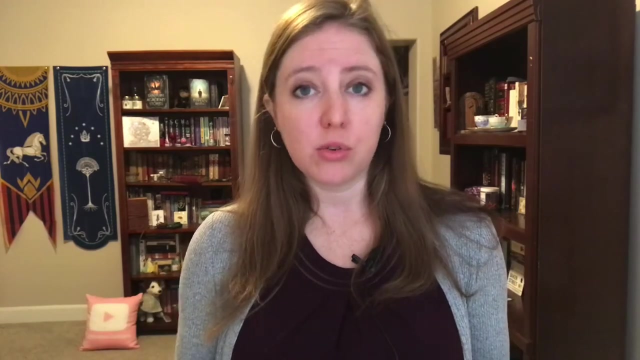 changed about what's being mocked, then that is going to be satire as well. Very often satire will nod at itself. So you have Geoffrey Chaucer, who was in the Canterbury Tales making fun of the three estate system, and that was that men could only be in one of three social 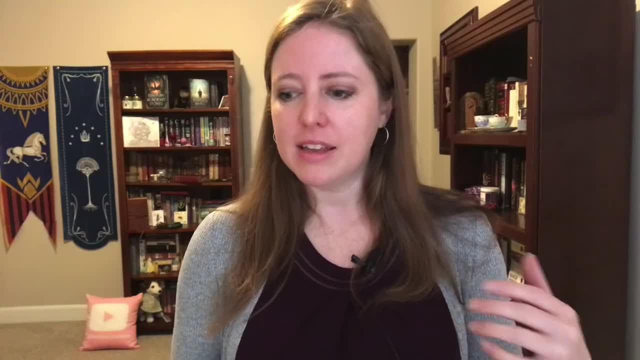 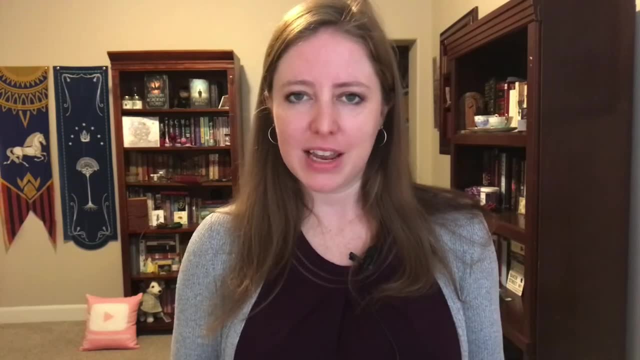 categories and Chaucer thought that was nonsense and he says in his general prologue: please forgive me for overlooking all, all degrees, but I'm not going to do that. I am not as learned as I ought to be and in Jonathan Swift's essay there is a 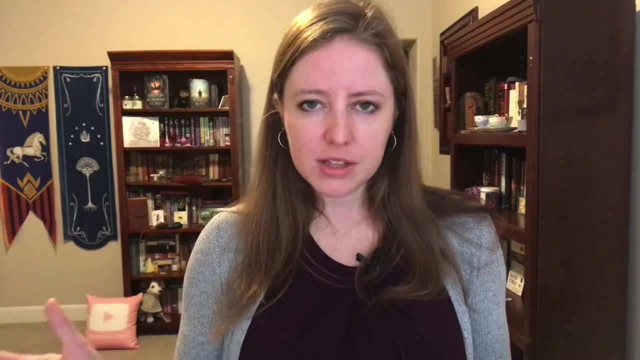 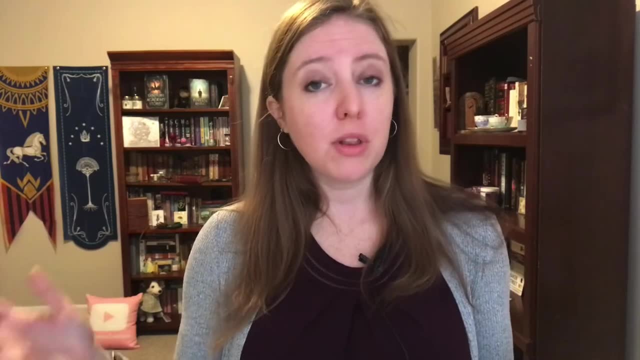 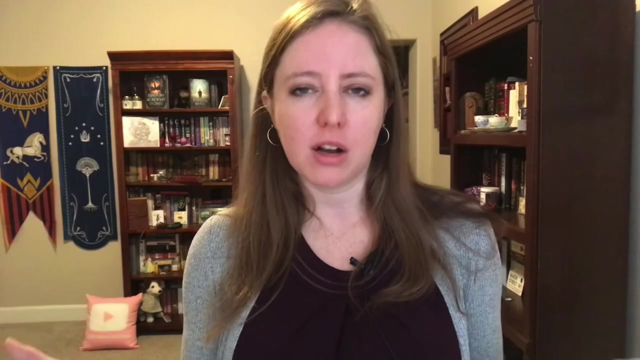 section that says: let's, let's try this insane project. he doesn't call it insane, but let's try this project, you know, because nobody's going to put these things actually into action. and then he gives a list of actual suggestions and he says: let nobody talk to me about these or other expedients unless you. 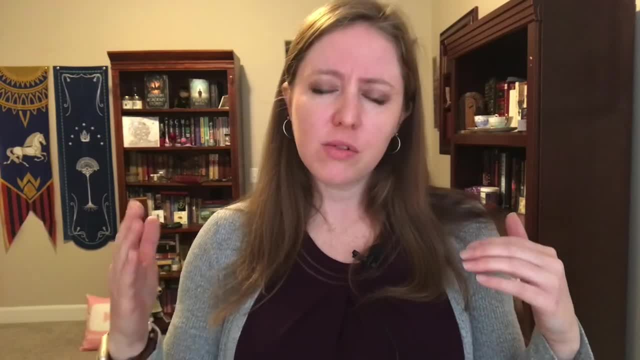 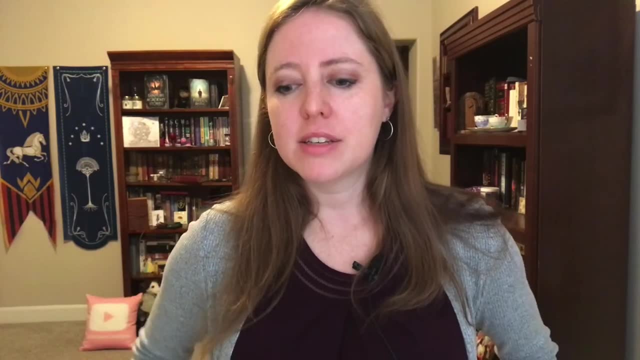 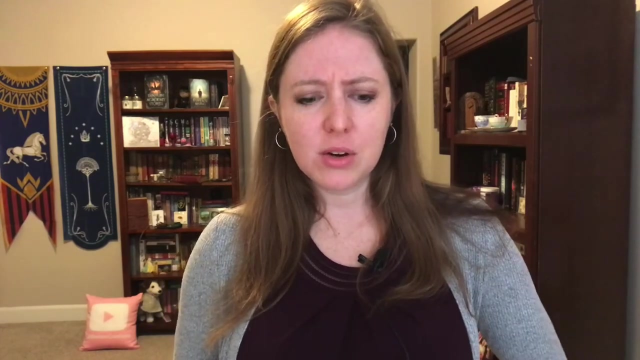 know you're actually going to try them. So look for those little hints that there is an actual suggestion hidden in there somewhere, and once again that means that it is most likely a satire. So if you have any questions, I know this was quick and I went a little over two.